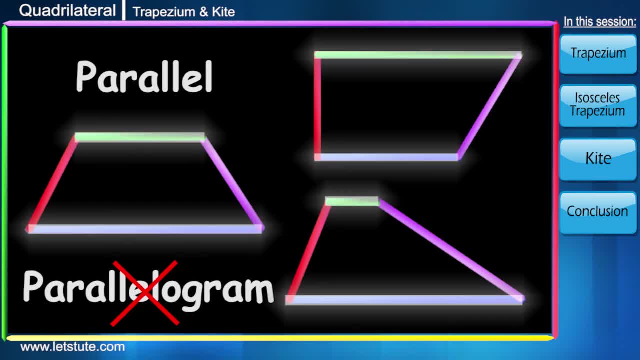 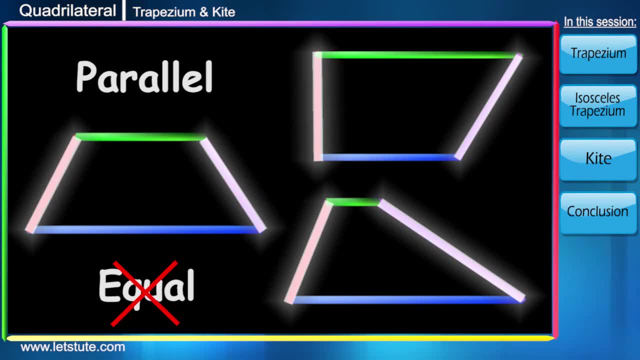 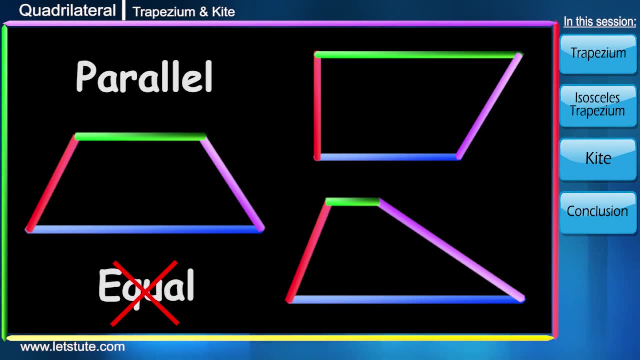 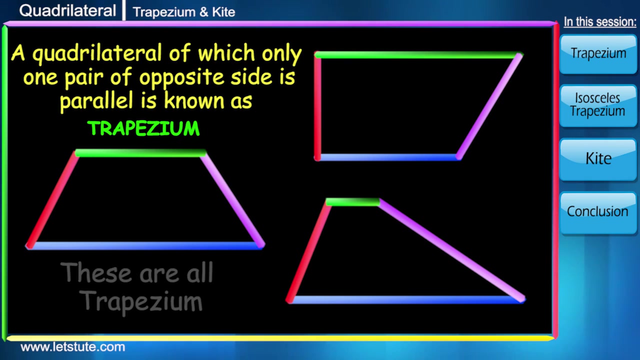 although one pair of opposite side is parallel, they are not equal in length, which restricts other pair of opposite sides from being parallel. friends, do not get confused between parallel sides and equal sides. okay, in geometry a quadrilateral was only one pair of opposite side is parallel is known as. 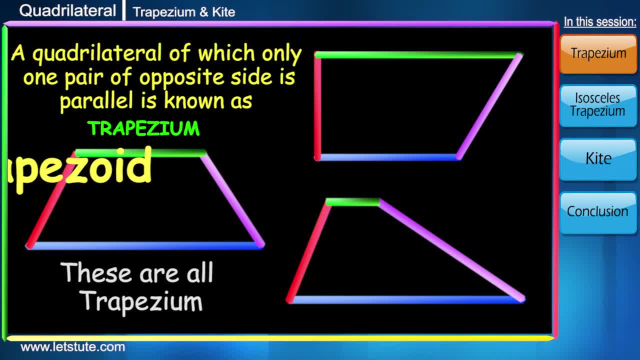 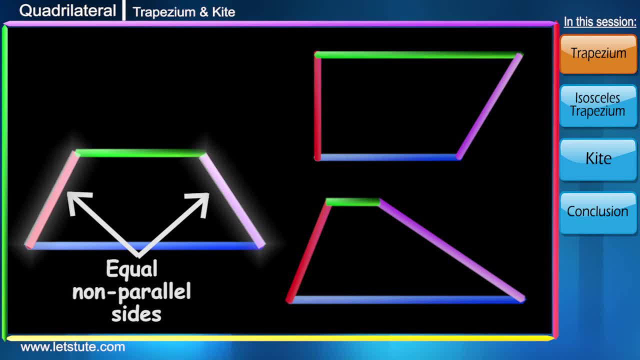 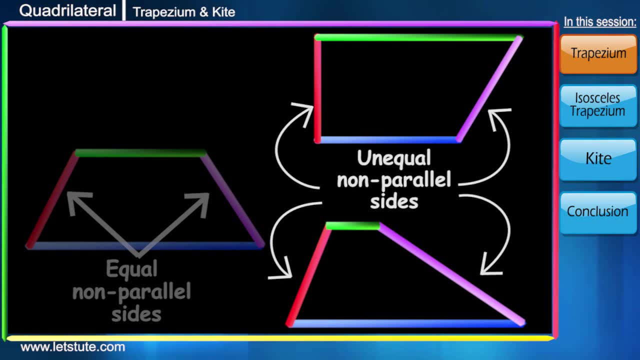 trapezium. some call it as trapezoid as well. these non parallel sides may be equal, like in our first diagram, or may not be equal, like in other two diagrams. basically, there are only two types of trapezium. when these sides are equal, we call them isosceles trapezium. 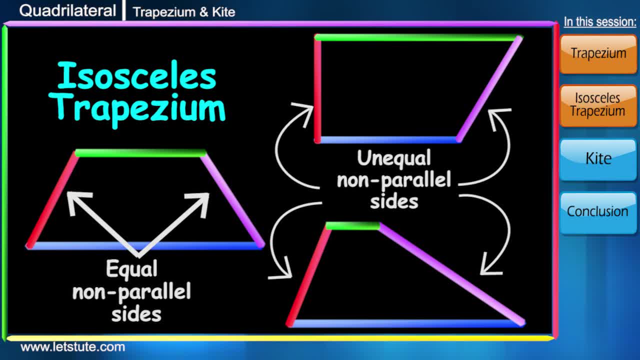 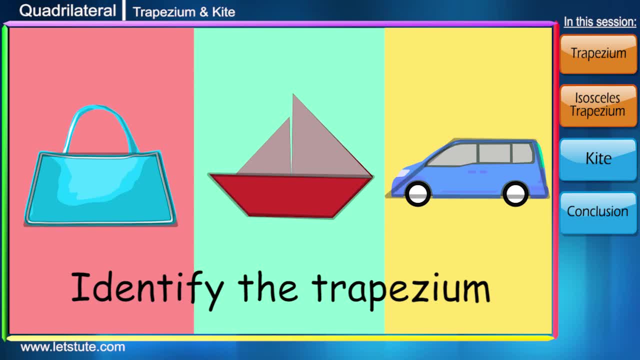 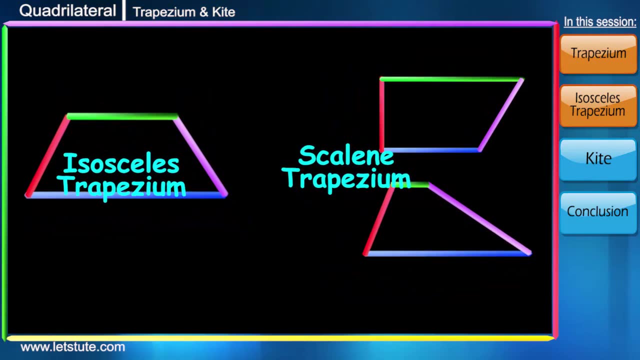 when they are not. they are simply called trapezium, or we can say scalene trapezium. here are some real-life examples of trapezium. since it is a bit different shape than that of a parallelogram, so even its properties will also differ, like opposite angles will not be equal, and 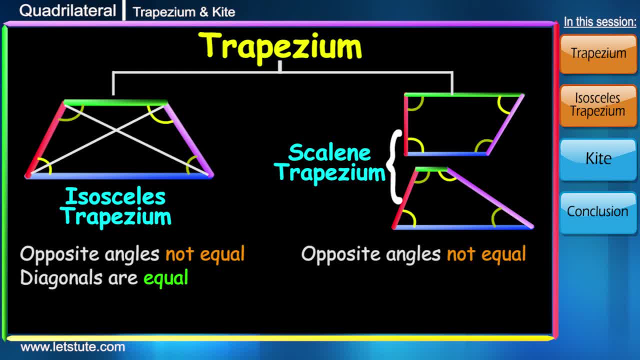 diagonals may be equal, as in the first case, that is, in isosceles trapezium, or may not be equal, like in any other trapezium. in isosceles trapezium, adjacent angles made by non parallel sides are equal. 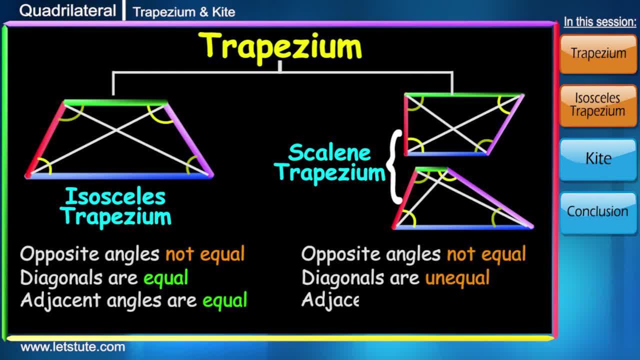 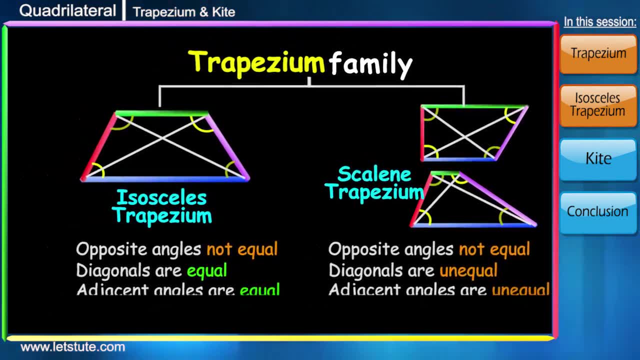 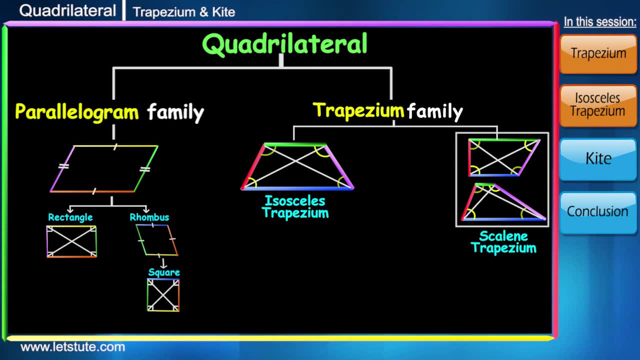 they are not in any other trapezium. they are not. so this was all about trapezium family. till now, we've learned about two families of quadrilaterals. if anyone asks you to recognize a shape belonging to these families, i hope you will be able to. now there is only one family left, the kite family. we've all. 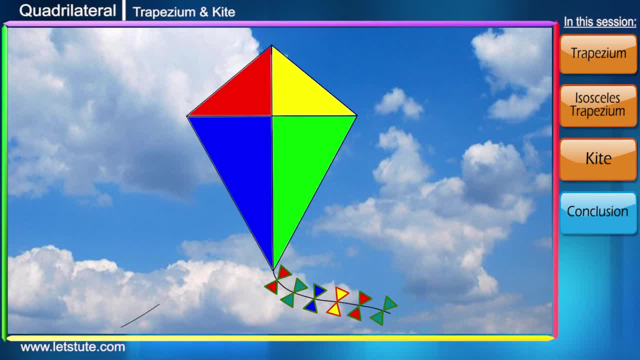 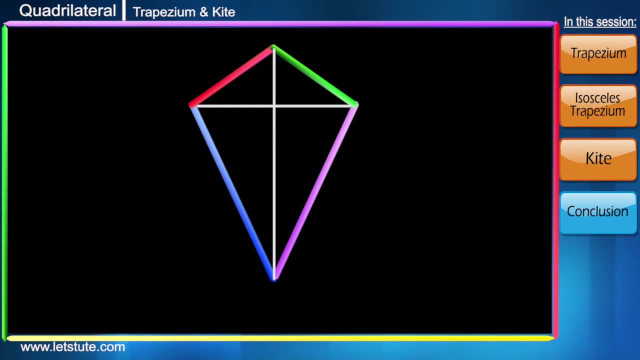 seen a kite flying in the sky. in a kite there are two main sticks which helps in the kite flying. friends, try to make the shape of a kite along with me with these Mikado stick and write whatever you observe. I've made three kites and all of. 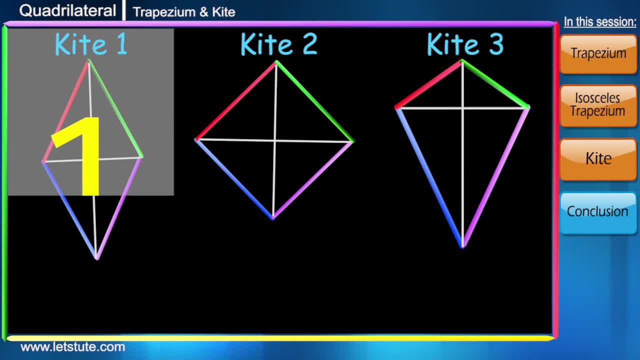 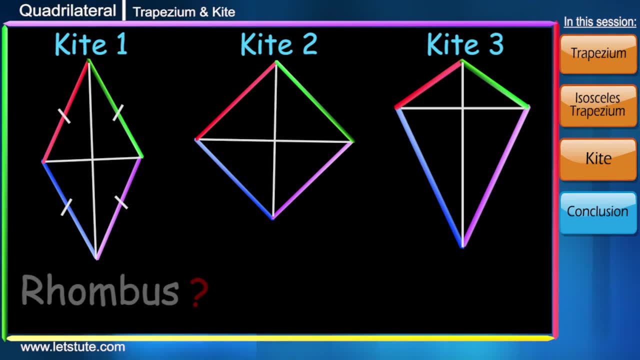 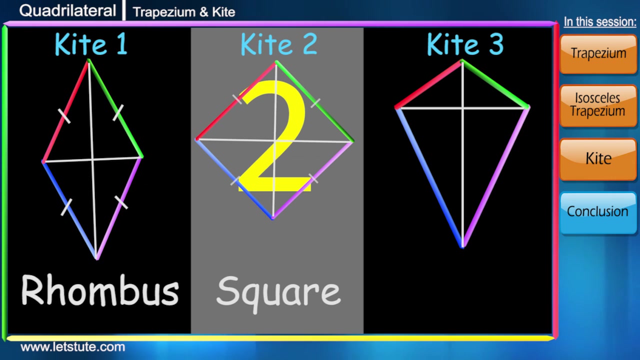 them are a bit different from each other. see my first kite. all its sides are of equal length. can we call it a rhombus, which we have learned in our previous session? if all the sides are equal, they have to be parallel, so it becomes a rhombus, right? it could have been a square also, like my second kite, as it. 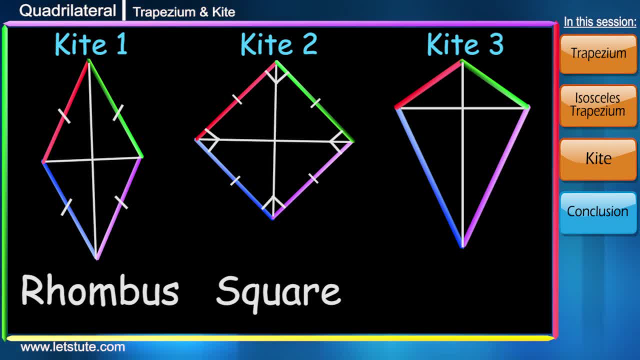 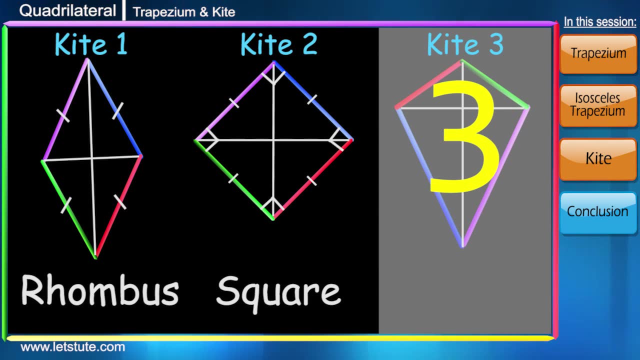 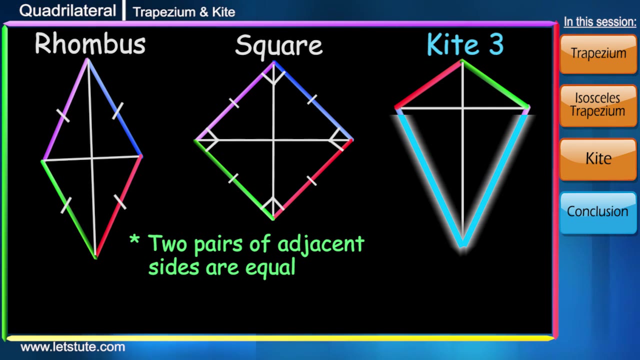 makes 90 degrees of angle at the corners. simply if we rotate or flip a rhombus or square, it looks like the shape of a kite, only right. my third kite is a very special one. we haven't seen such quadrilateral till now. it's both. the pair of adjacent sides are equal. this is. 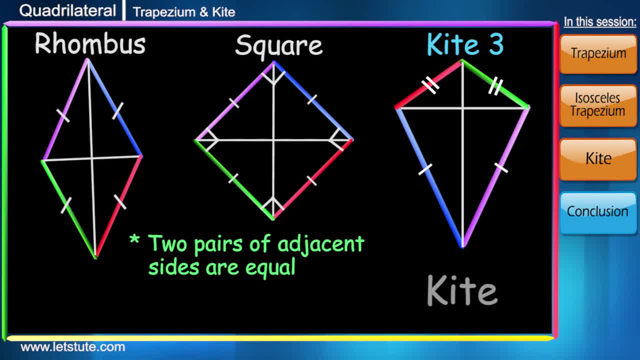 one of the criteria for a quadrilateral to be a kite. there is one more property which is only found in kite is that we can see its diagonals are perpendicular to each other. precisely speaking, it's one of the diagonals is a perpendicular bisector of other. why you must be. 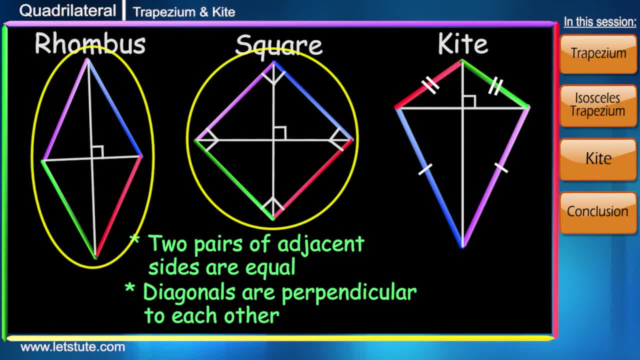 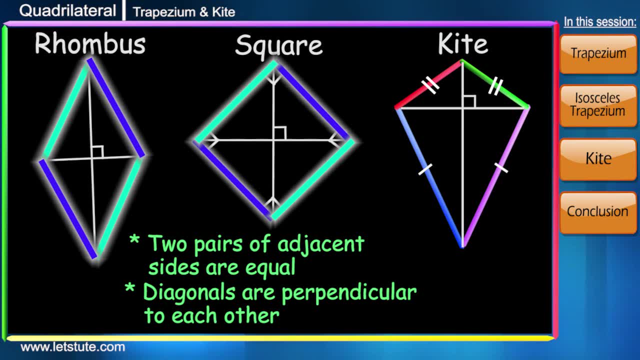 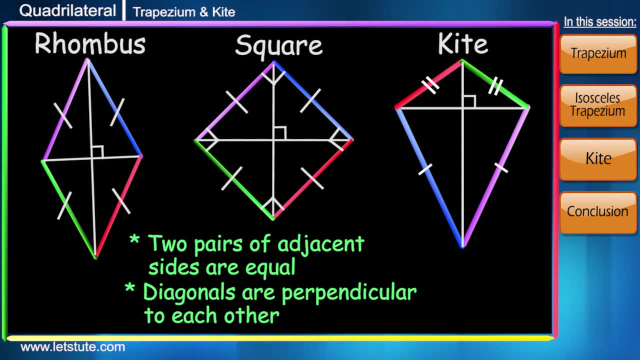 thinking that the square and rhombus belong to the family of parallelogram because both their pairs of opposite sides are parallel. Yes, you are right. in a rhombus or square, since all the sides are equal, so doubt, even adjacent sides will be equal, as well, as their diagonals are. 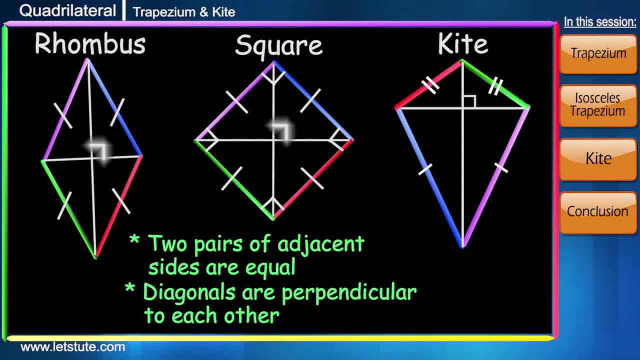 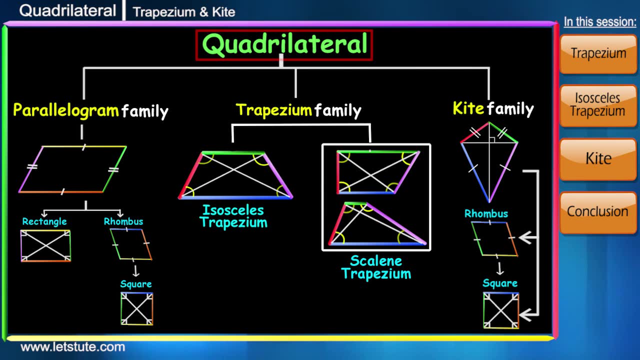 perpendicular to each other. therefore, they belong to both the families because they satisfy all the tradition, or you can say condition, followed by respective families. so, friends, this was all about the types of quadrilaterals. any other shapes which do not belong to these three families are simply called. 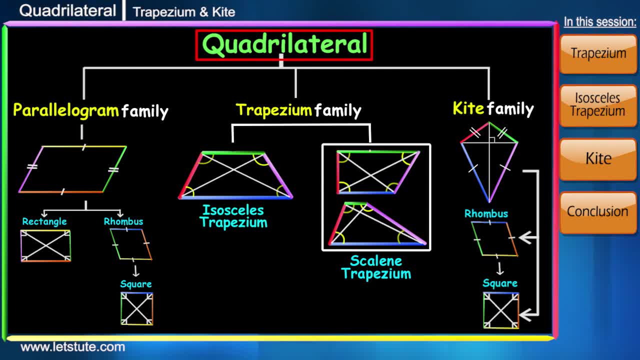 quadrilateral. only broadly we can say that a parallelogram, trapezium and kite are the family name or surname and the figures which come under these families have their different names. rhombus and square are in a relation with two families, parallelogram and kite. all these